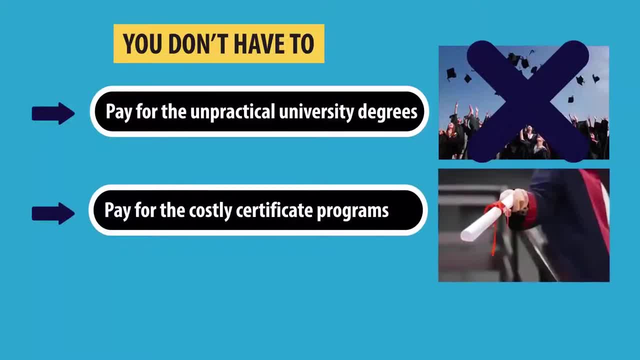 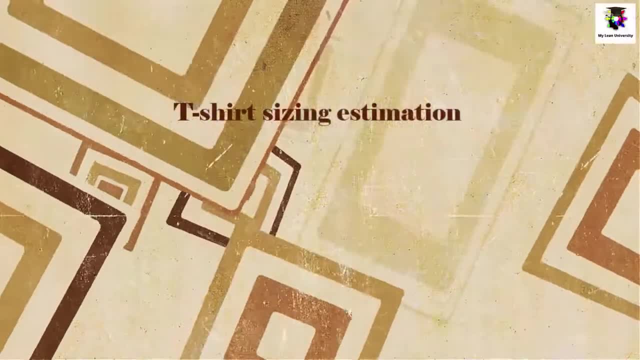 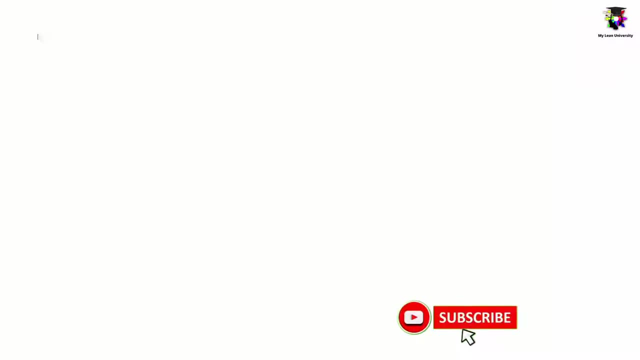 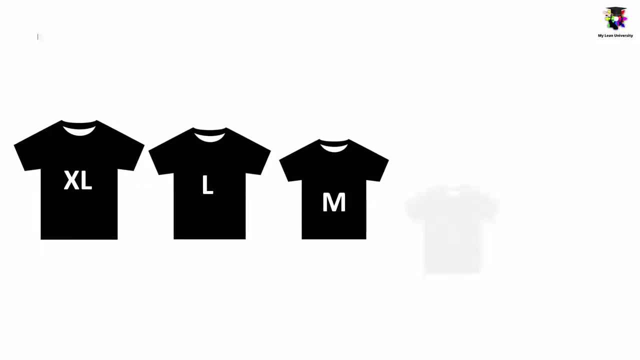 subscribe to My Lean University, which is my initiative to deliver free and quality professional education to your screen. There is an another method of estimation of the user stories when a quick and a rough estimation of a massive backlog items is required. In this technique, the size are estimated in a t-short: sizes ranging from XL, or extra large, to XS, or extra small, which. 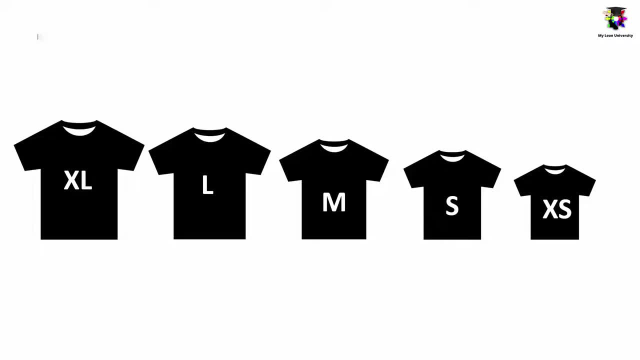 simply denotes the size or number. So what does these sizes mean? Let us see the two outlier sizes. XL or extra large represents the complex and lengthy walk which requires more time compared to the other user stories. XS represents very simple user stories where no complex walks are involved. This 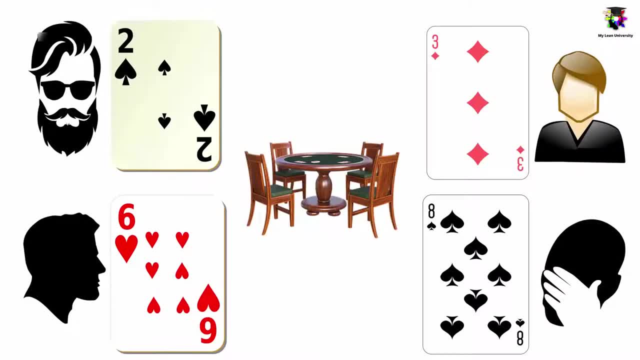 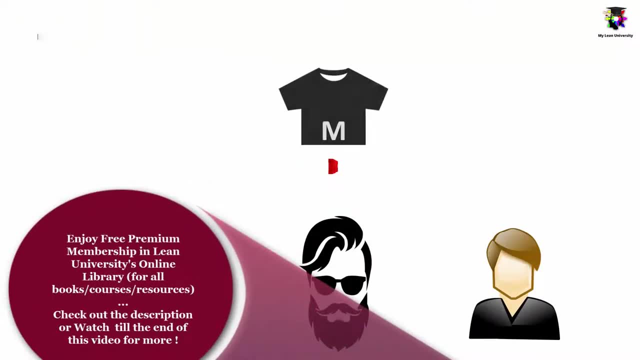 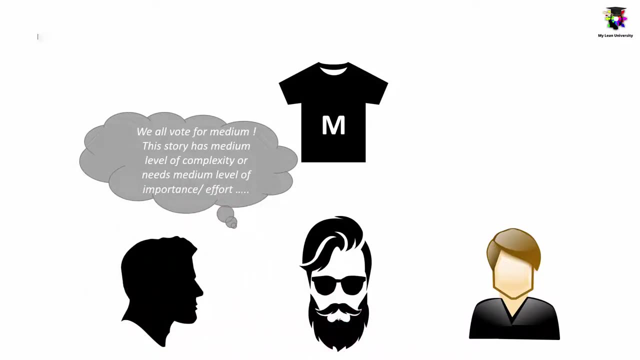 estimation technique is kind of similar to that of a planning poker. The team assigns a size to the user story. If the size offered by each estimator is the same, then that would be considered as the final size. However, in case of mismatch, there is a discussion to reach the consensus before arriving the final estimate. 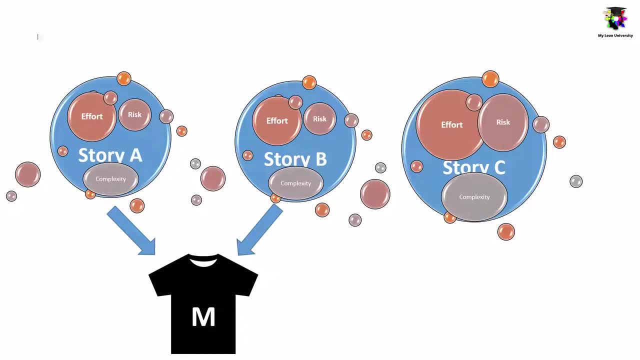 The size assigning process is relative to each other. for example, in this case the function of complexity, effort and risk or uncertainty for backlog item is similar, So let us suppose it was assigned to the medium or M size. the other backlog item required a much. 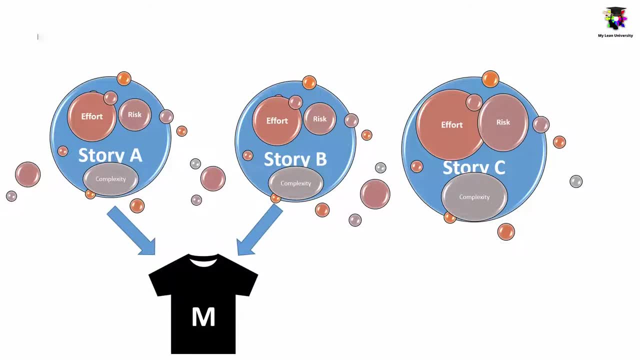 larger effort, larger risk and complexities. hence we can relatively assign it to a larger t-shirt group. so here we see that t-shirt sizing is relative to each other, which is of course the basic approach of every agile estimation approaches. so t-shirt sizing was relatively easy in the next. 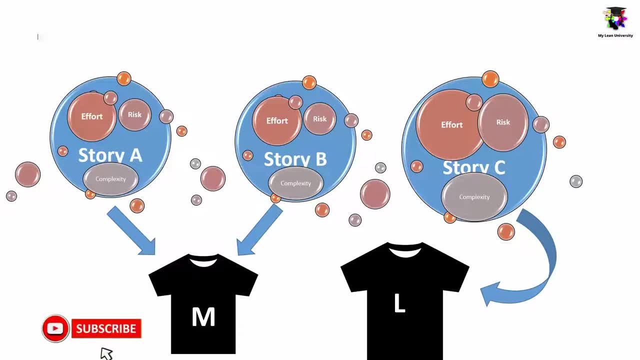 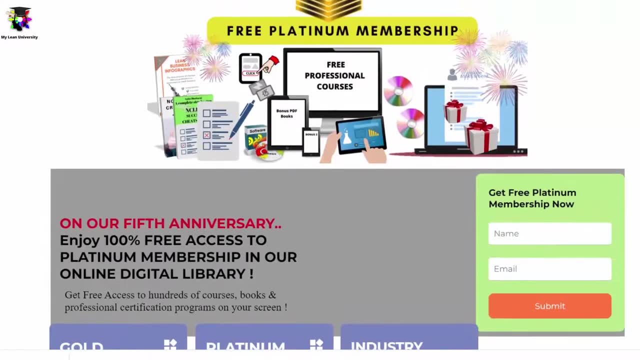 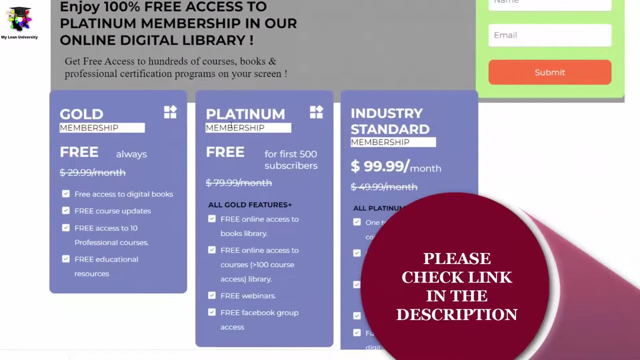 lecture we will see some other few techniques of estimating. Спасибо user stories of the backlog items. before ending this lecture, let me remind you to join my lean University's premium membership and enjoy a total free asks for limited time inside my lean University's online library and get tons.